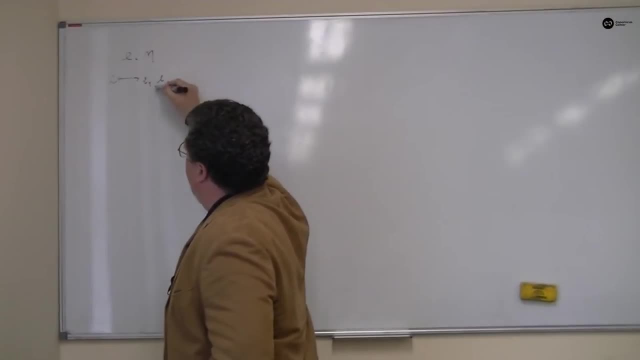 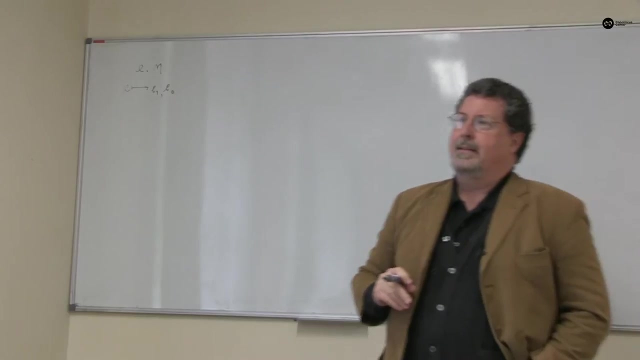 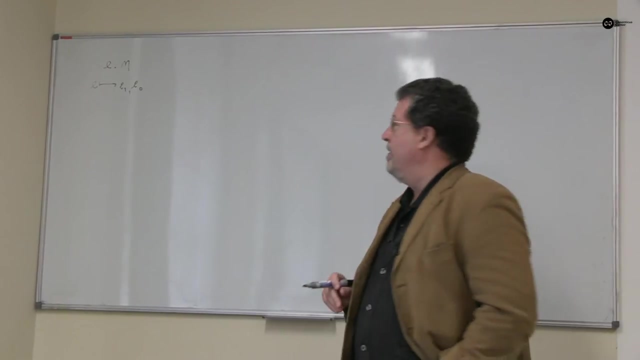 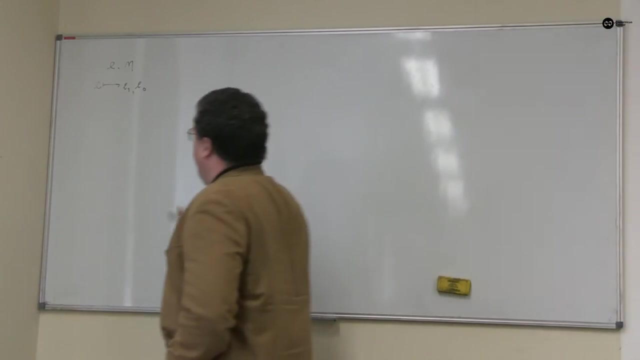 I can divide it up using unpairing into its components E0 and E1. I can do left unpairing and right unpairing. These are effective functions. I can do that in terms of prime number factors in the number E And if I have some kind of effective predicate of natural. 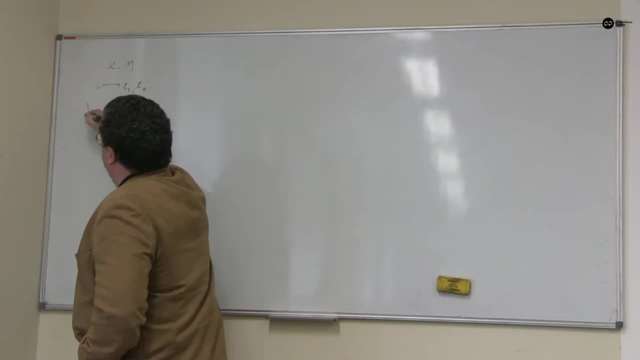 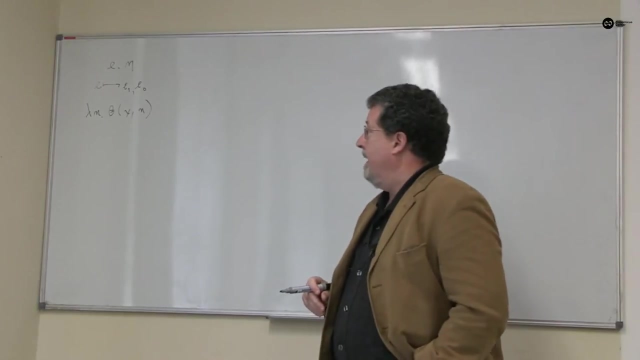 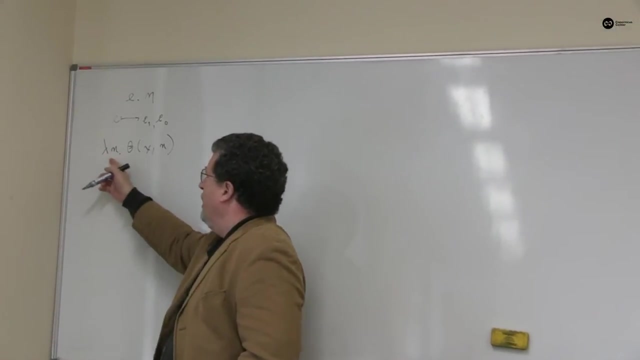 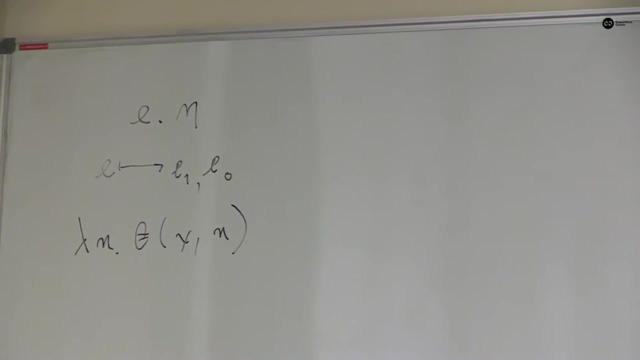 numbers and I can do lambda abstraction onto it and I get an effective predicate of numbers, now effective in X, where I'm now talking about. in X I output the procedure that accepts N as an input and produces theta XN. I'm going to use these little pieces of notation from 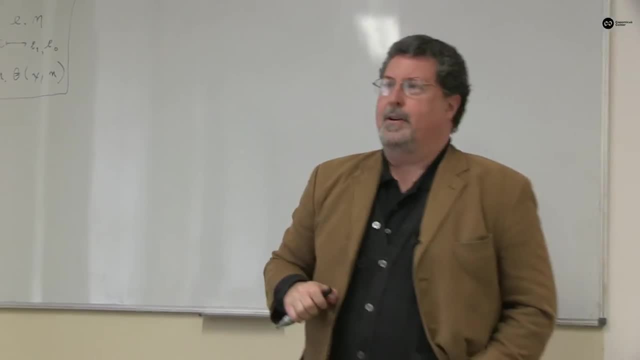 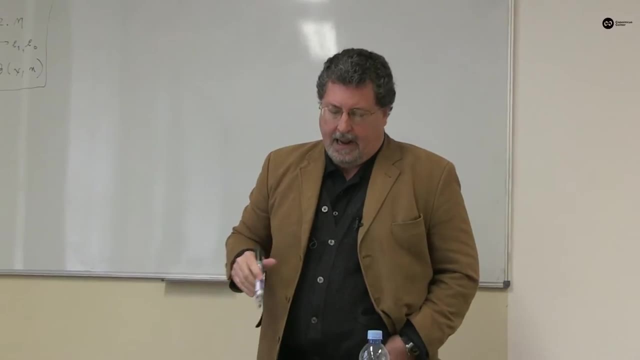 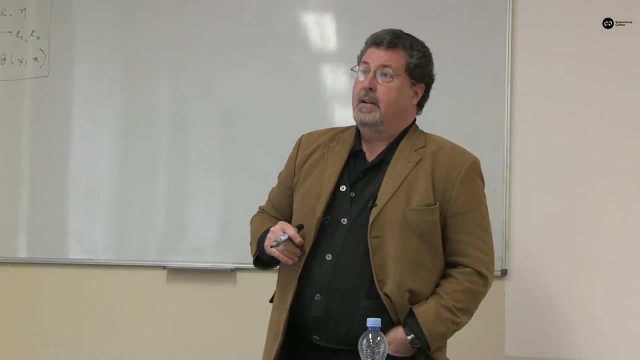 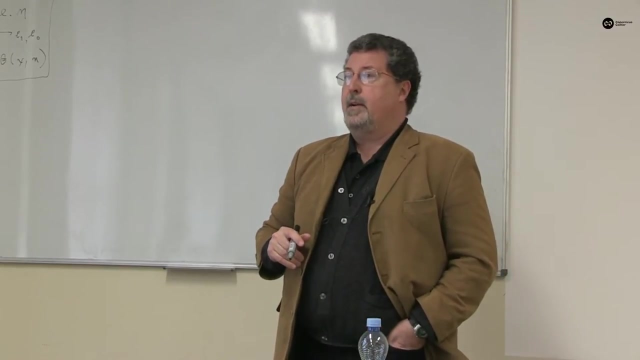 elementary algorithm theory or elementary recursion theory, effective calculation theory. The proof proceeds almost entirely from the intuitionistic version of what you could call the T-scheme. It corresponds in a rough way to Tarski's T-scheme from his great paper The Wahrheitsbegriff, And I might write it this way: 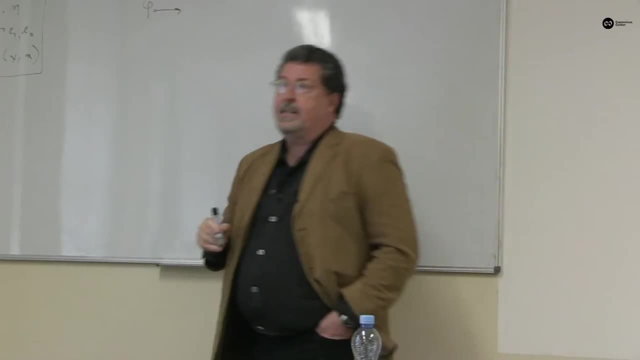 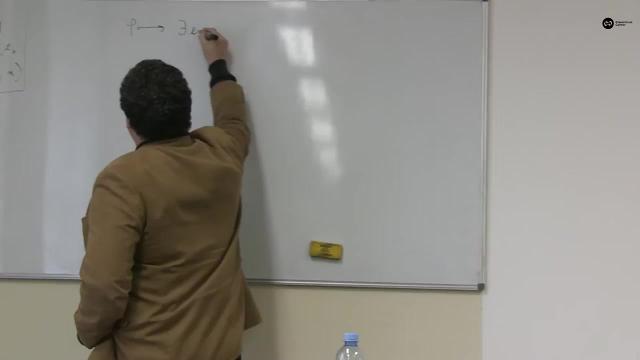 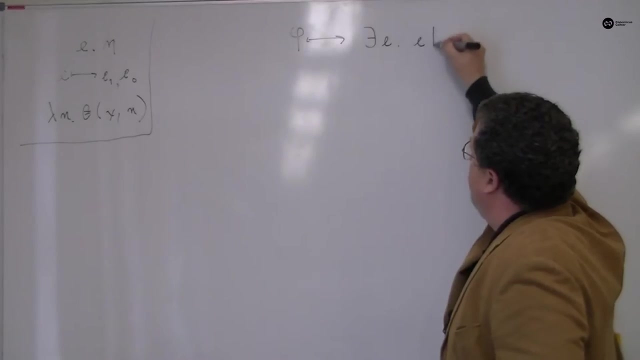 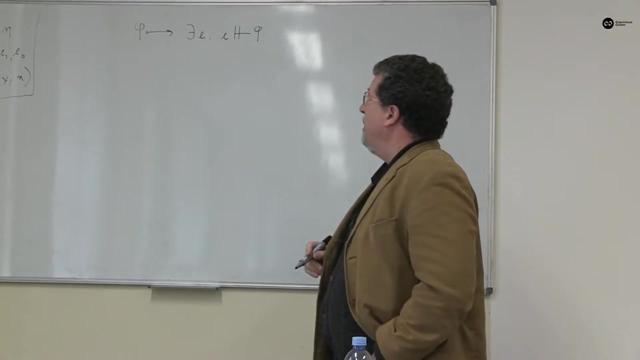 Phi is a sentence, or a sentence in parameters, and it holds if, and only if, there is a natural number, E, that encodes a construction such that E constructs phi, And one of the basic ideas of intuitionistic mathematics is that such a relation. I'm writing, I'm using the 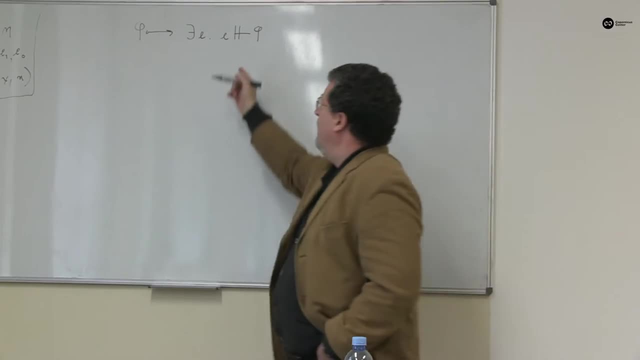 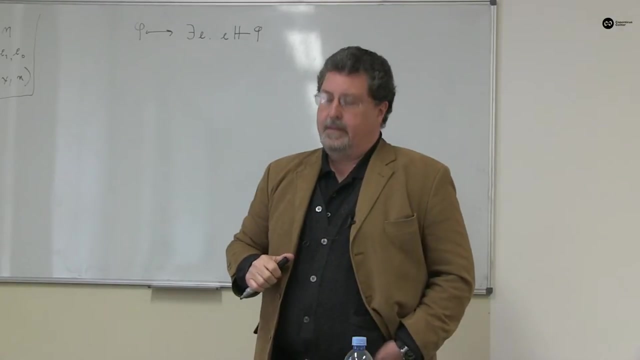 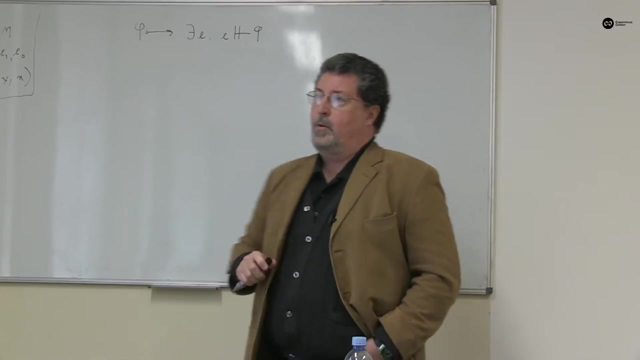 forcing symbol, But I'll just read it: constructs. Such a relation can be defined recursively and it can be proven to exist. It's an idea that goes back to Ehrenheitink, Kolmogorov, others And I only really need. 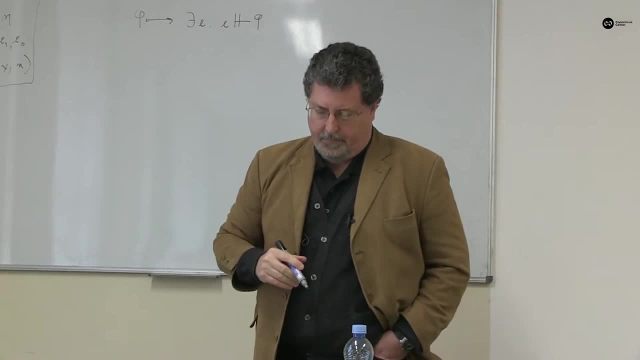 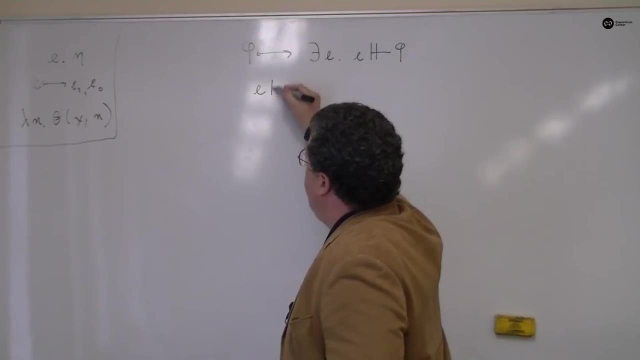 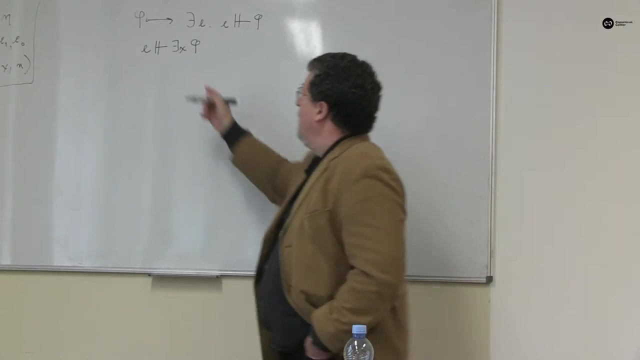 two clauses from the definition of constructs. They're both familiar. I shall say that natural number e encodes a construction of. there exists an x, phi, where here I'm thinking of all my variables throughout as ranging over natural numbers. That's not necessary. 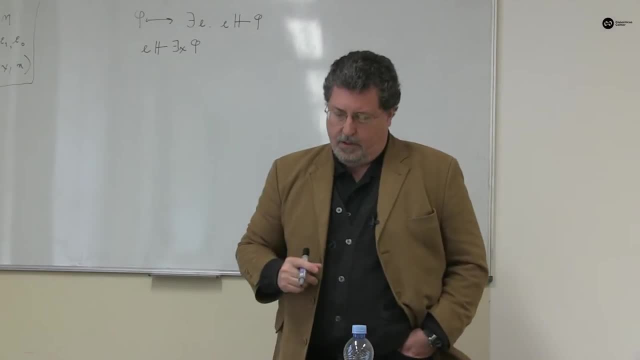 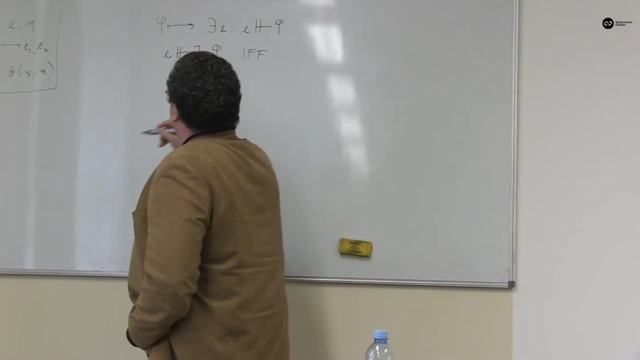 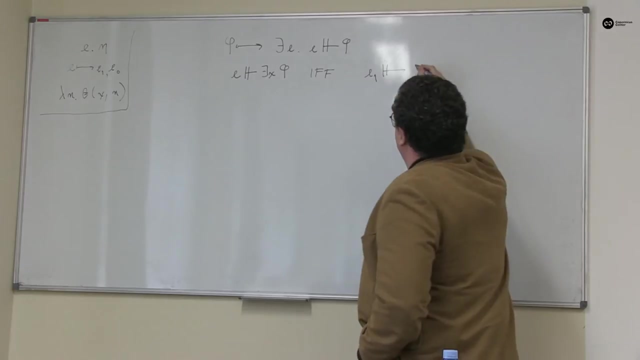 but for the present purposes it will be no limitation. This holds if, and only if. I can do unpairing on e and e1 encodes a construction such that phi holds of e0. and just to be perfectly definite, here are the natural numbers. e0 is a natural number, Just write that. 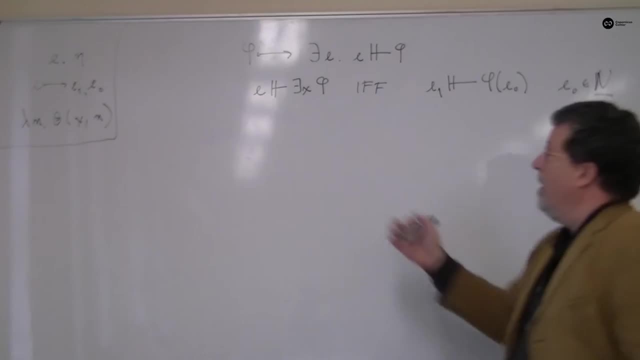 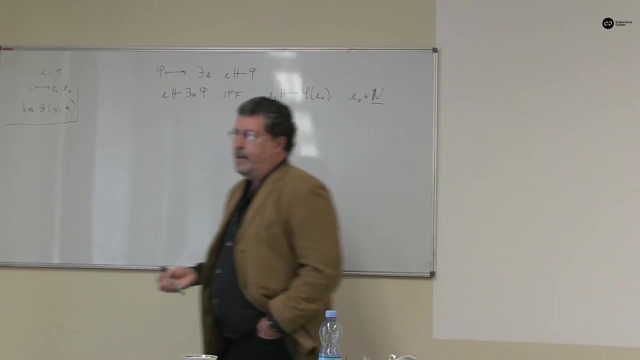 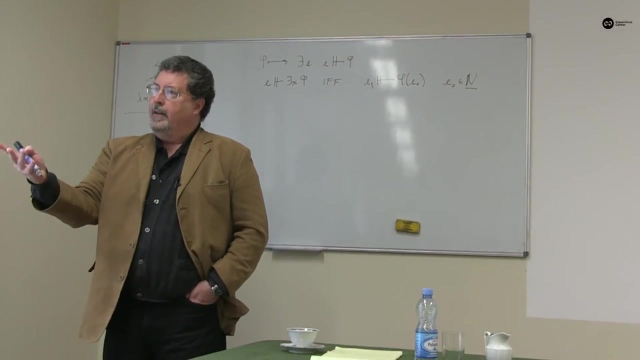 there to remind ourselves that e0 is a natural number. And so I have a construction that constructs an existential statement if, and only if, that construction can be effectively broke apart into two sub-constructors, if you like, The second of which is a construction. 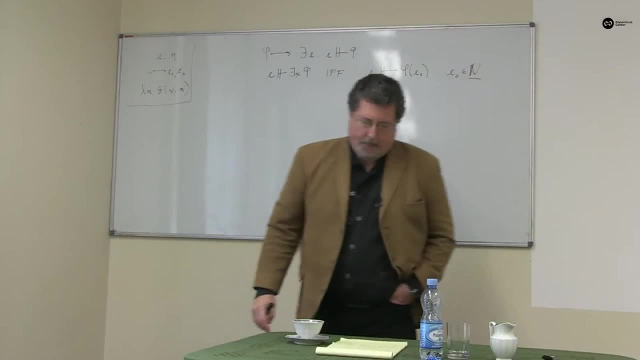 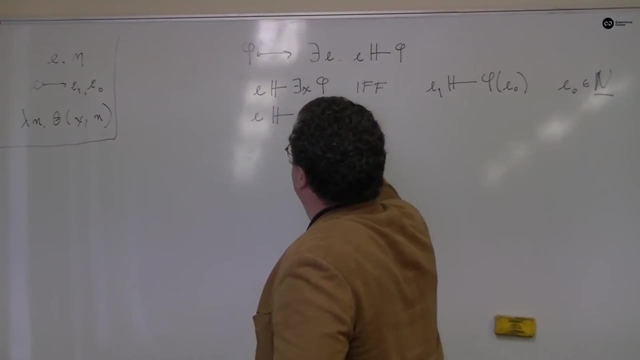 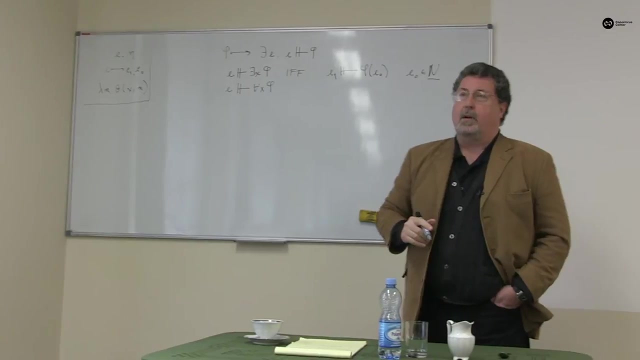 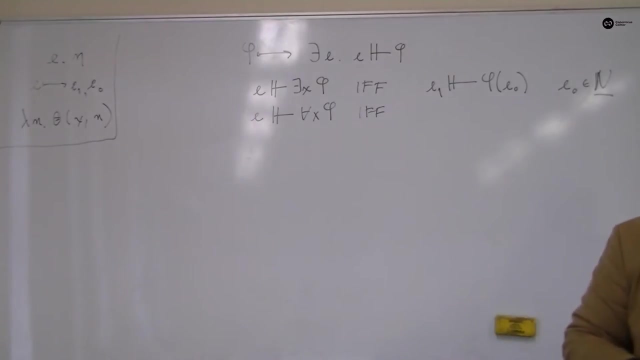 that phi holds on the first, which, And then secondly, e encodes a construction, a universal claim about natural numbers. By the way, I intend phi here to hold with respect to parameters and not just searches, If, and only if, we think of e as encoded in. 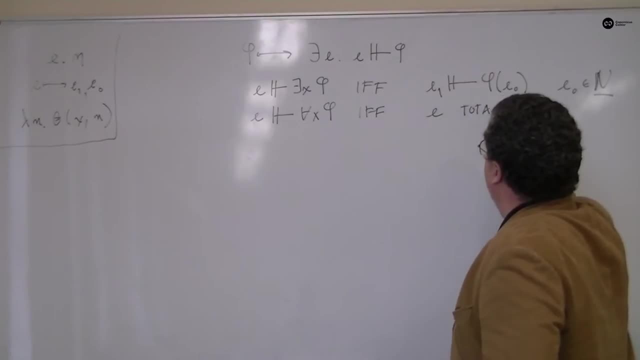 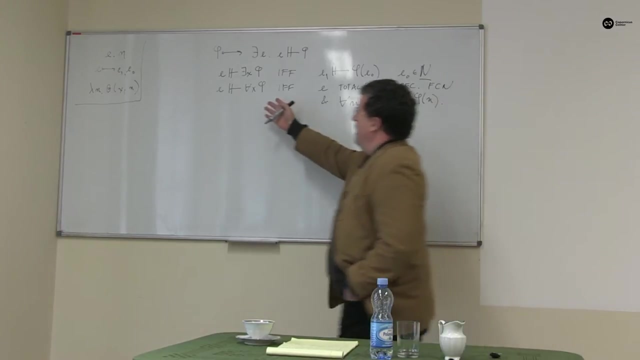 a total general recursive function And for all natural numbers, n. if I apply e to n, I get a construction for phi of n. This is an idea that you find in some of the later papers of David Hilbert, for example when he explains what it is for such a statement. 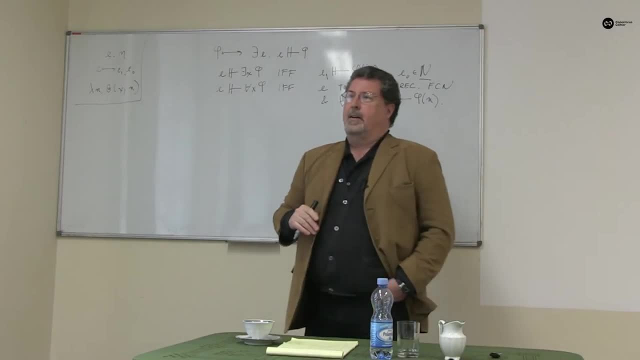 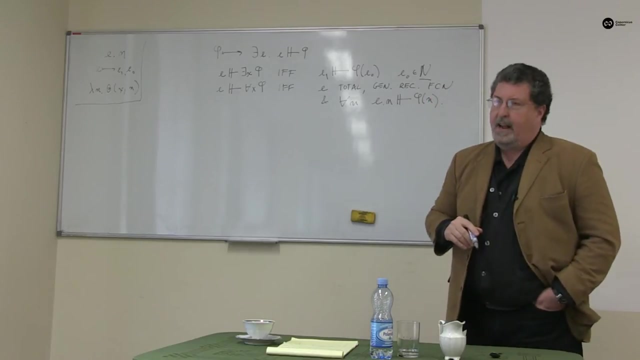 to be true in a finitistic fashion, That is, that there is a procedure available on the basis of which I can enumerate proofs- finitistic proofs of phi applied to each natural number, n. So it's a function: I input a natural number, I get a proof out. proof of phi of n. I should 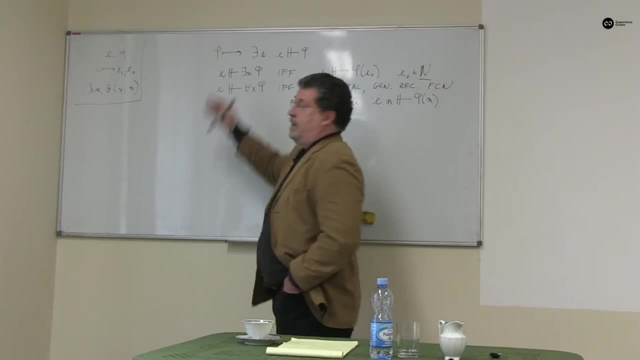 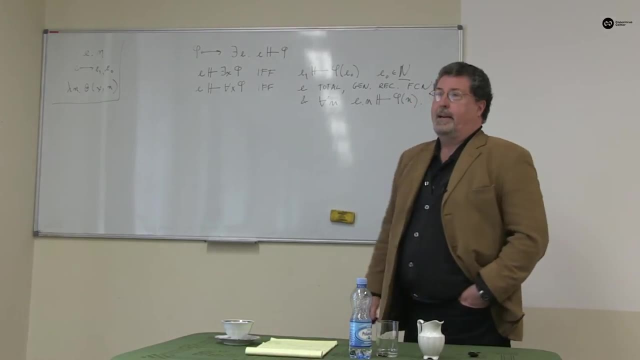 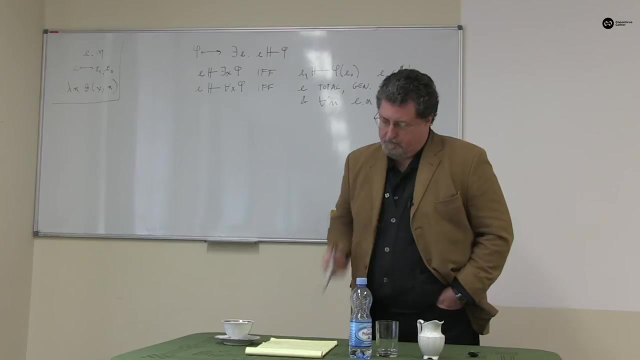 be careful though: I'm not thinking of this as a concrete proof relation. I'm thinking of it as an abstract relation between- we can encode everything and call them- between numbers, but at least between numbers and parameterized formula. And now I'm going to. 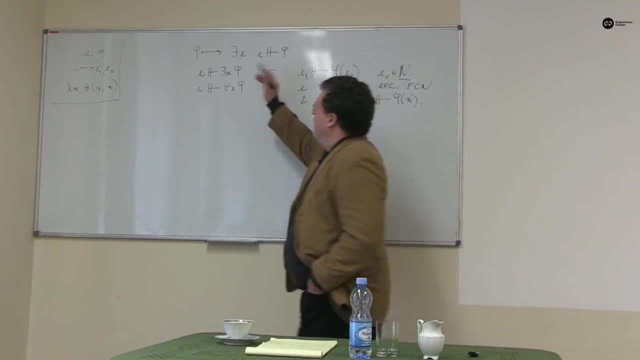 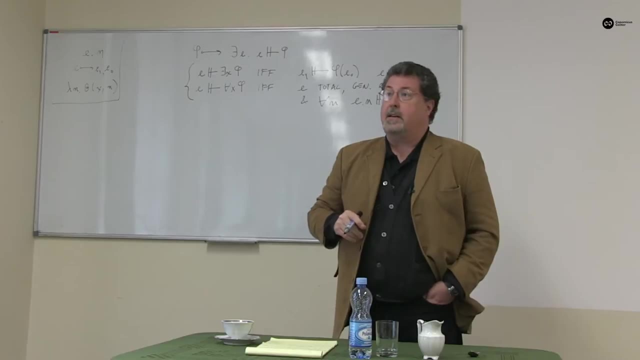 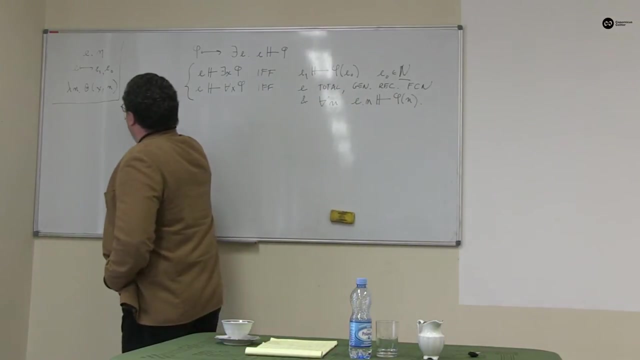 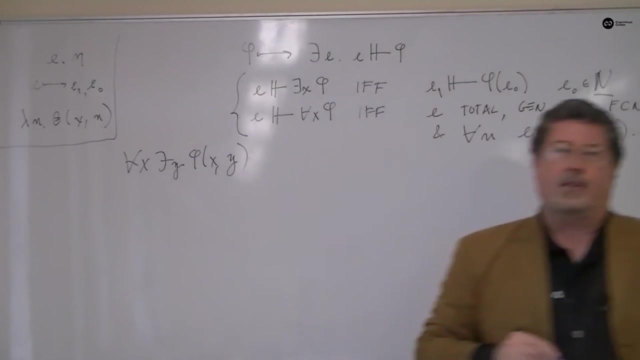 begin to show from this claim and this partial definition that Church's thesis is understood by intuitionists. So let's start out with the claim that phi, perhaps in parameters, defines a total relation over the natural numbers. For every natural number x, there's a natural number y such 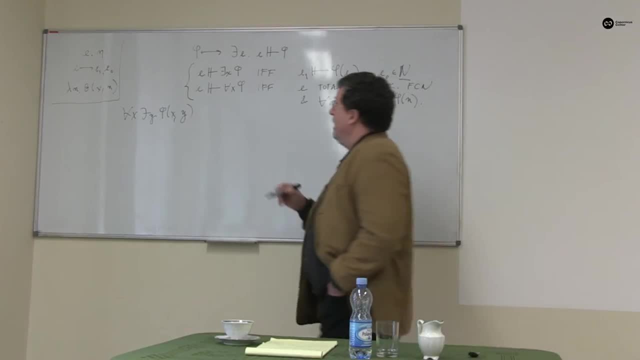 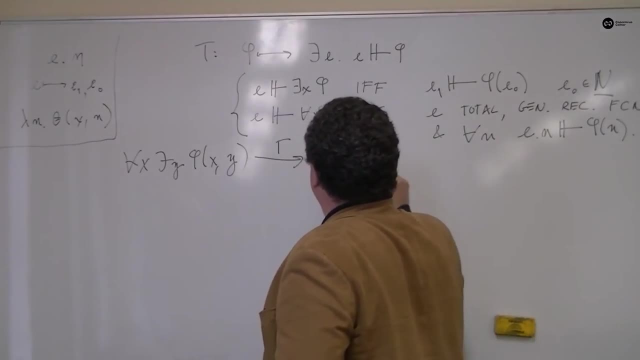 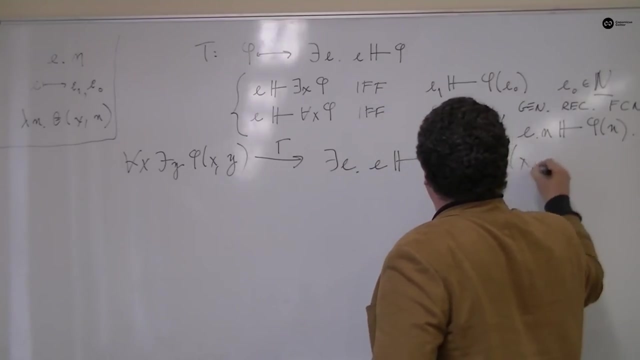 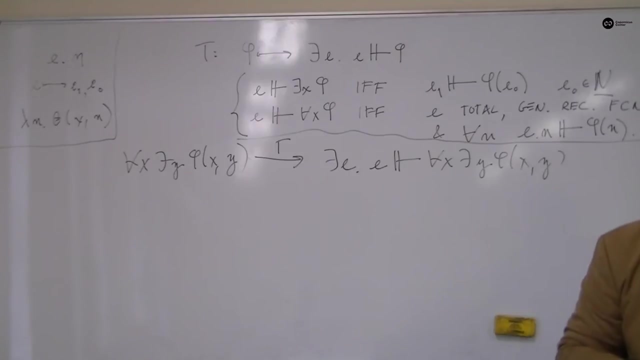 that phi, x, y, Then by the t-scheme. it follows that there is a construction that constructs this parameterized expression. Let me draw a line here separating these. And then it follows: here is a universal quantifier of numbers from this part of the definition. 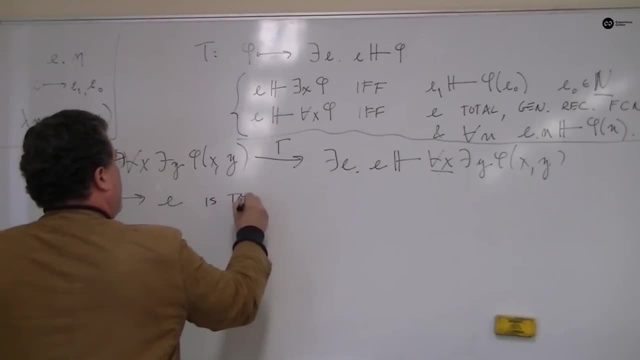 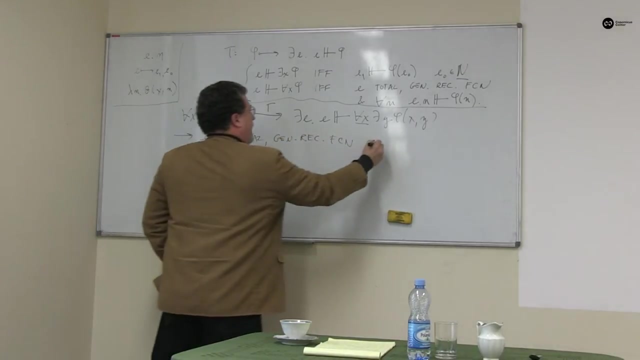 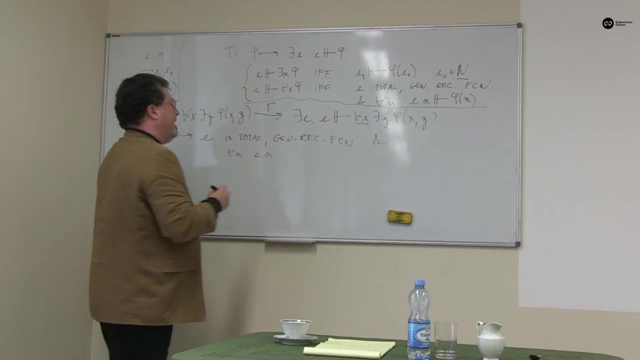 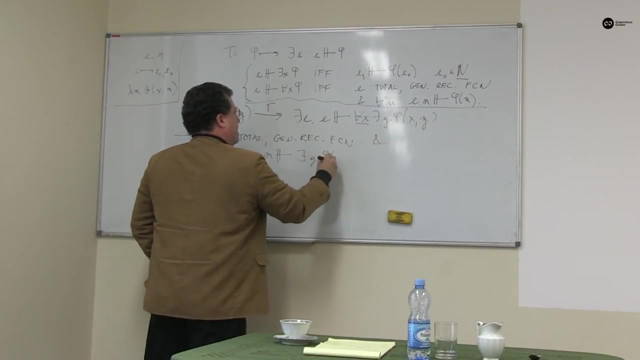 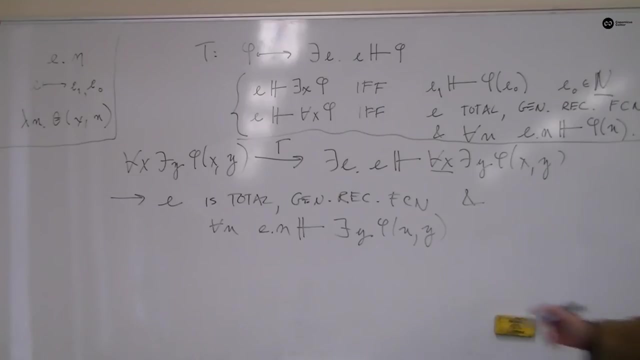 that e is total general recursive function of numbers and that phi is a function of n And for every natural number n. if I apply e to n and take the result, it gives me a construction of this, with x replaced by n, And I continue to reduce. I now have a complicated 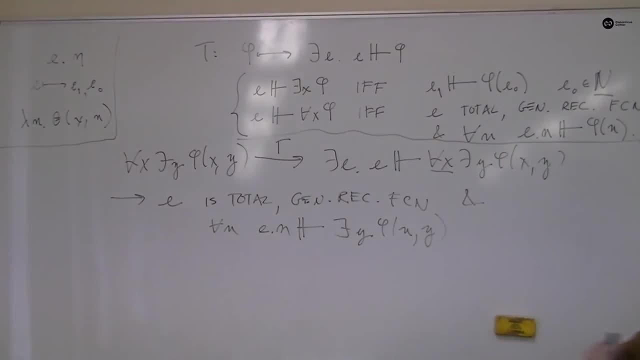 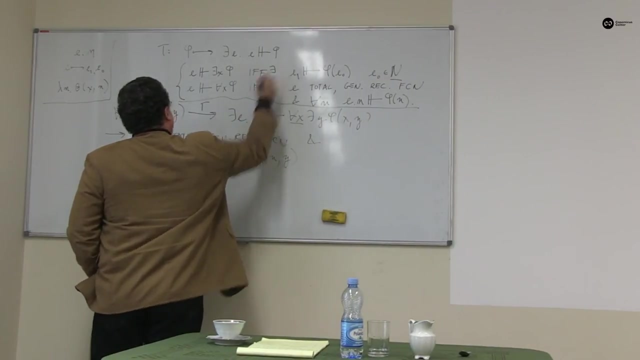 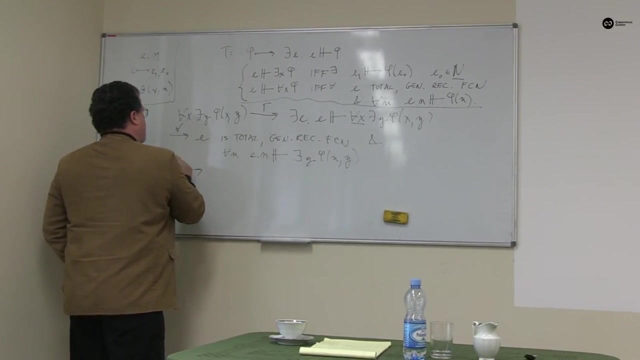 term standing in the constructs relation to a parameterized existential statement. and so if we call this one the for-all clause and this one the existence clause, this holds by for-all And then by the existence existence clause We're going to get: e is total, It's. 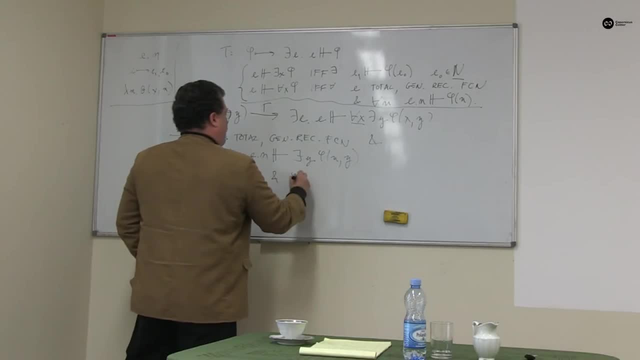 general recursive And for all n. now I apply the unpairing operation e, n 1, write written like that Constructs e and n, Q e n 1.. The variable here can be divided into n-thh and. n-thh and n-thh, All right, written like that constructs n, n, 0,, n, x. That is not all. How about the noise compared to the number of numbers? If we take this, say, m's, m-h and. 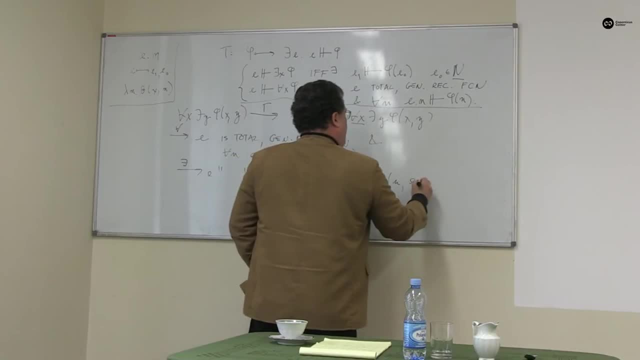 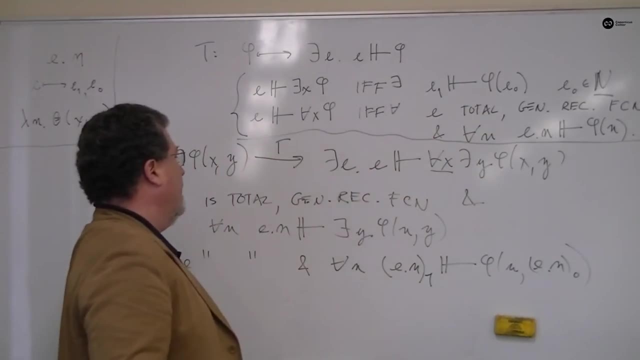 n are Religion and耶's. and which number does that? then we'll get t z-th. let's get that phi n e n zero. So I've just applied the existential clause here into the parametrized statement. 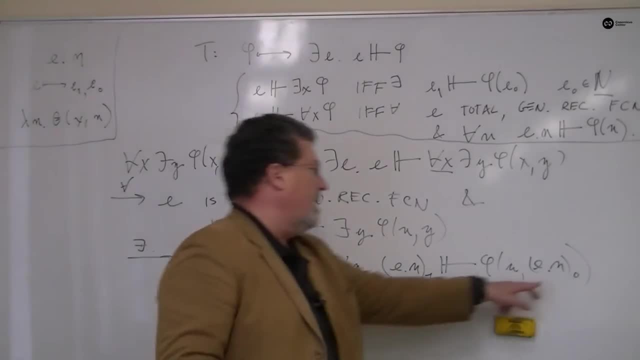 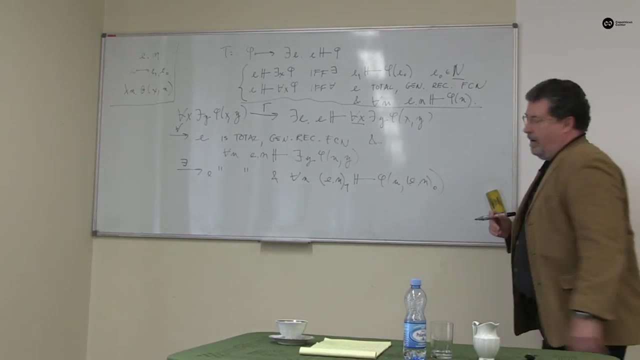 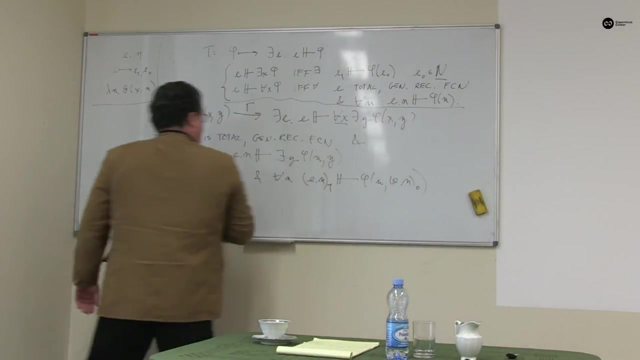 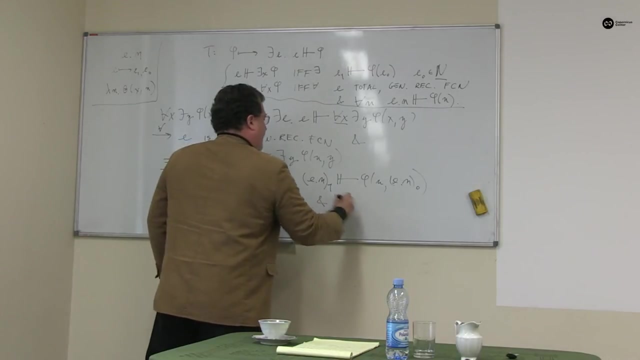 And I know that the second component of this constructs the formula instantiated on the first component. And now I'm going to apply the T-scheme in reverse. going this way, I now know that e is total general recursive and for all n, my T-scheme tells me. 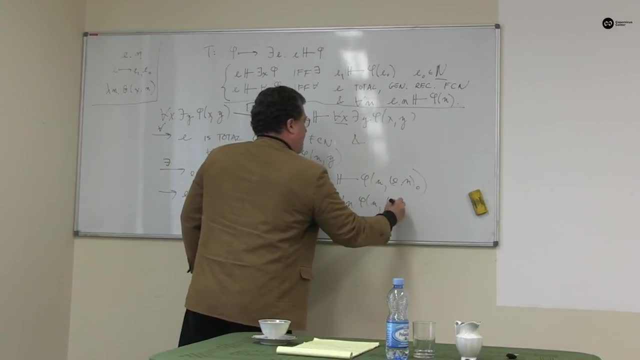 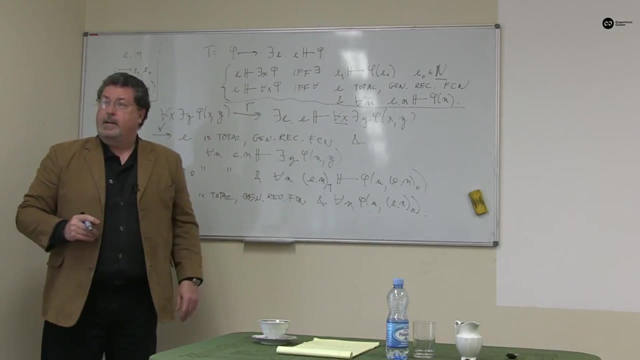 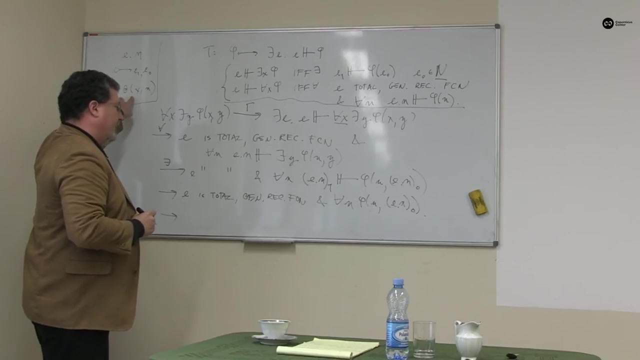 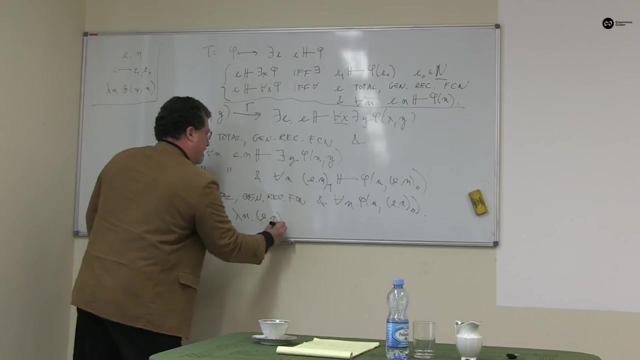 I can drop this off. phi n e applied to n zero because this was a formulation that was assumed in parameters. And now I'm going to do an abstraction. I'm going to let g encode the procedure that gives me lambda n e, n zero. 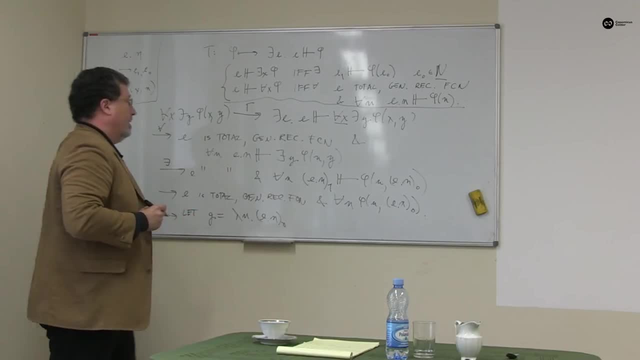 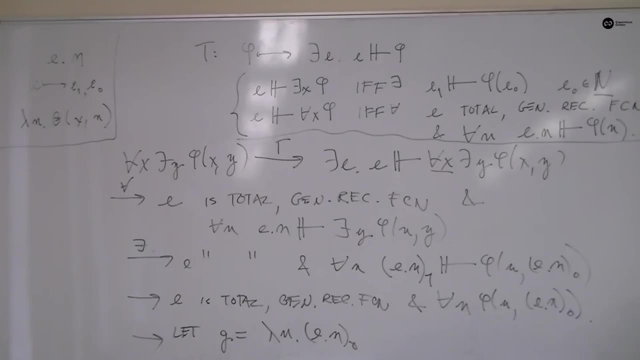 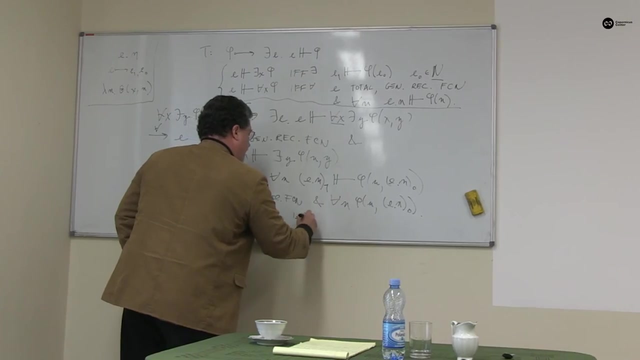 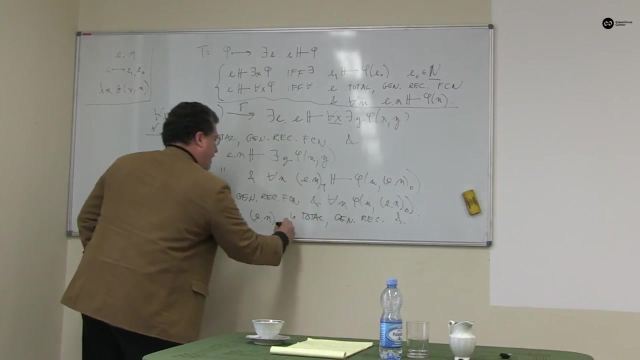 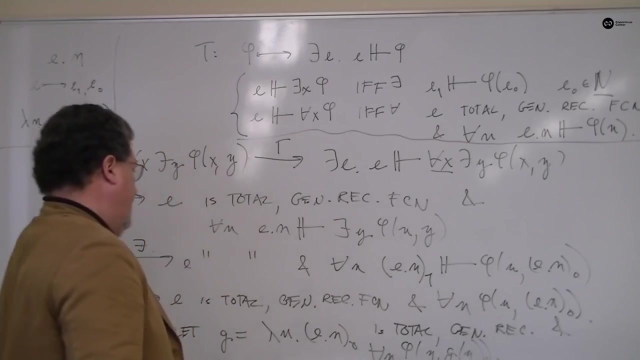 I assumed that into functional context I can perform abstractions and recursivity is being performed. Thank you being preserved. Zero is total. We assume that EN is total. So this thing is total. It's general recursive And we now have for all N phi, N, GMN. So, putting it all together, 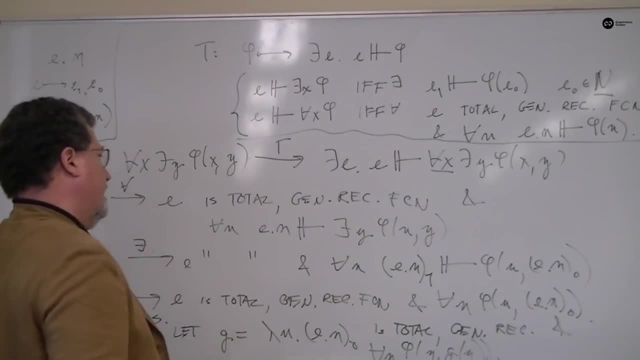 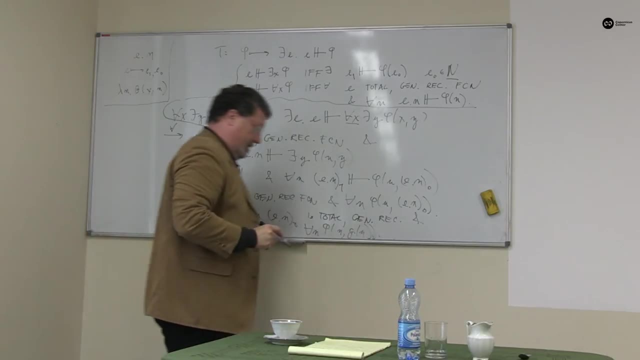 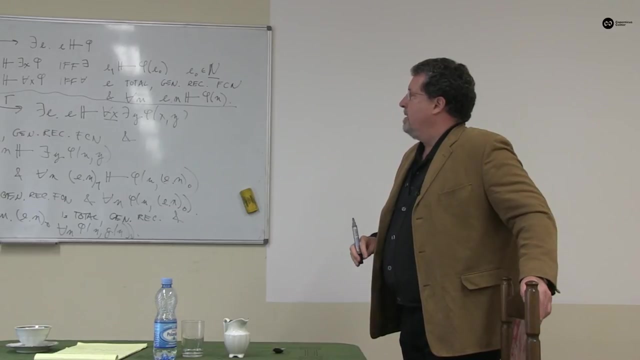 here I've just used abstraction, Here I've used the T scheme. What do we have putting it all together? Start with this assumption: It is machine-free, computability-free, perhaps. statement: for every natural number x, there is a natural number y, such that phi, xy, What's?